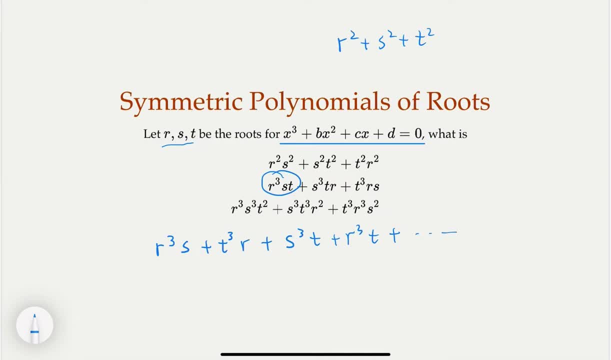 know, or all other combinations, right? You need to compute it in order to be symmetrical. If you remove any term like this, it won't be symmetrical, right? Because it's missing this term. All right, So it turned out that, and we learned that. you know, we're not going to be able to do this. We're going to. 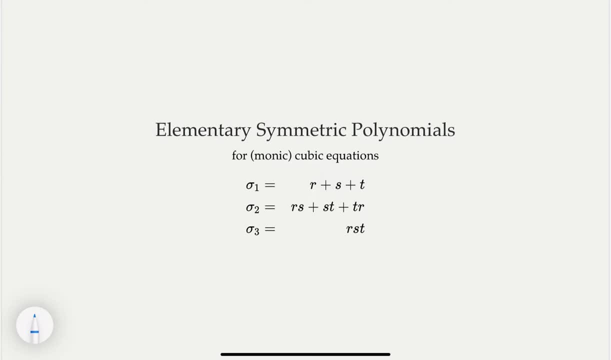 get the elementary symmetric polynomial where we, for the three roots right, R, S, T- This is sigma one, which is we take just one of the roots and then add them up. For sigma two, every time we take two, you know from three there's three choices- right And then add them up And for. 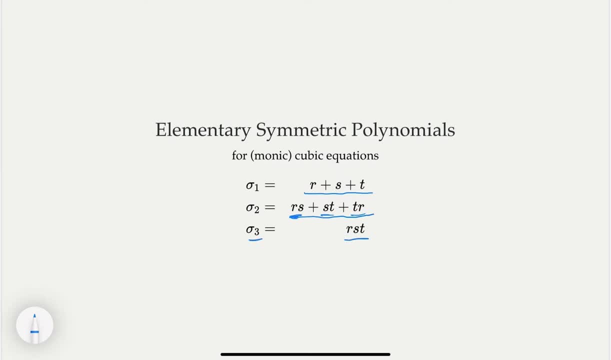 three, we choose three. There's only one way to choose three, That is, you know that's three, Right, And then you add them up for three Right Now, when you access the solution called elementary symmetric polynomial- we learned in the previous lectures, right. 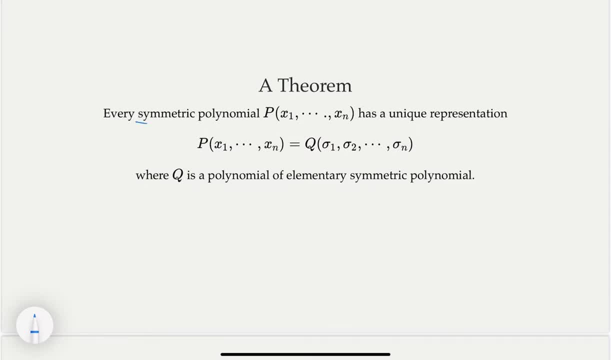 there's a theorem thing that for any symmetric polynomial there's a unique representation in terms of elementary polynomial. so by changing variables, you know, i can turn the original symmetric polynomial into symmetry in terms of the sigma 1 and sigma m. now in the cubic case, that would be sigma 1, sigma 2, sigma 3. there's some polynomial we need to find, and for any 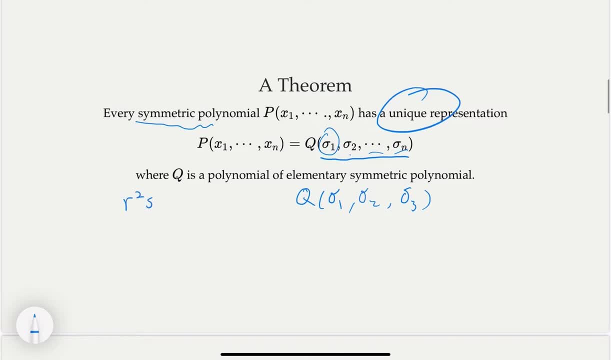 symmetrical polynomial, for example, the one we're going to look at right now. is this one right? so, basically, the theorem saying that there's a unique representation. we can find it, you know, but how do we find it right? so let's talk about that in order to do that, you know. 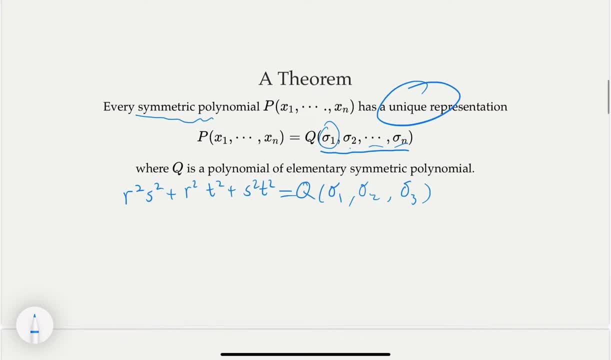 we're going to introduce some terminology, you know so, when we look at these terms in the polynomial right. so in generally, if there are variable, m variables, now each term is like raised to certain powers. so we're going to assume that each term- of course sometimes there may be- 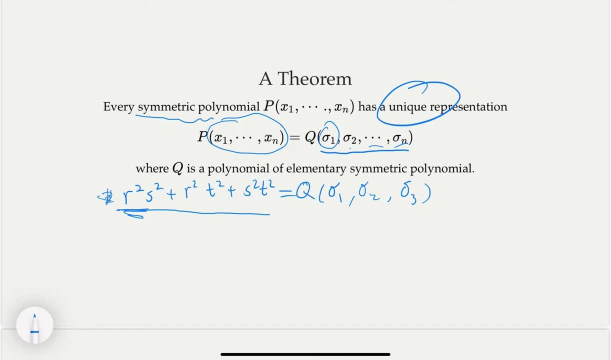 coefficient one or two. you know so some coefficient terms. each term is actually in. in general it could be a variable m one square. so, for example, if we take m one square and we take m2, it's m one square. so if we take m one square and we take m two square, and we take m two square and we take m one. 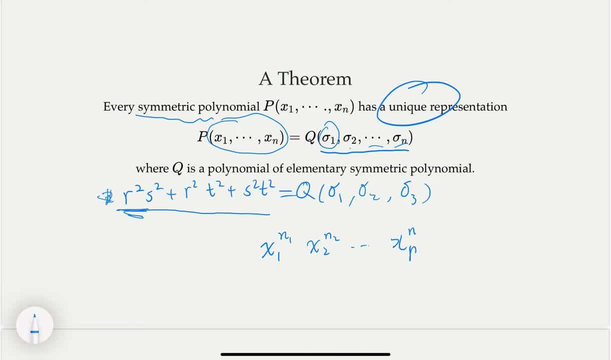 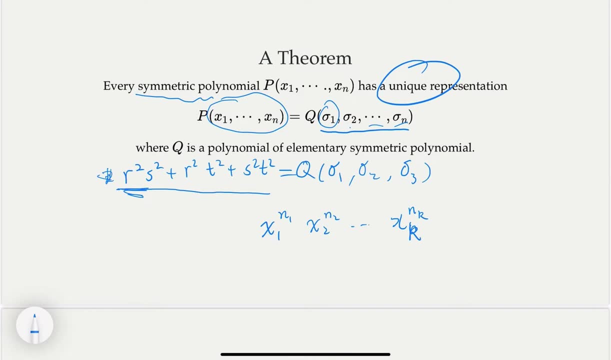 power, x two to the m2 power and x? n to the m- you know, m probably is not good word- this k to the nk's power, right? so in this case, right, there is a rst, and so each term, when we write it, this could become r, square, s, squared, but there's no t. but then we can make a t to the zeros power, right. 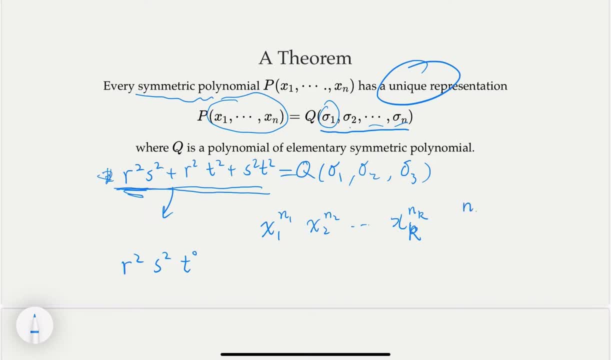 So sum of the n1,, n2, nk is non-negative right, Assume that is greater or equal to 0, right And the second term. of course you can write it as r squared: and s to the 0th power, t to the 2nd power. 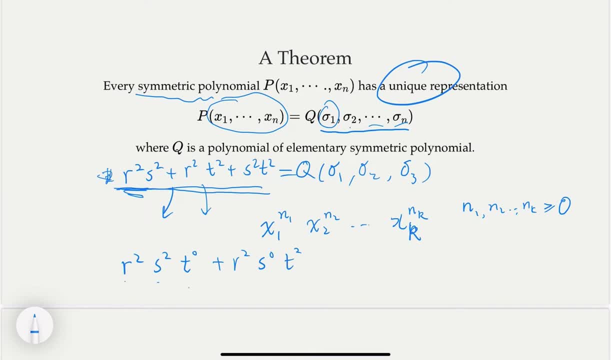 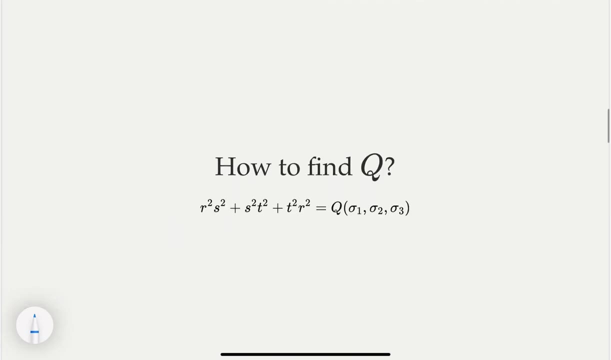 Remember, we always fix the order rst, x1 to xk, right, And then here, the last one would be: r to the 0th, power s squared and t squared. okay, So what is called the? you know how to find this right. q in terms of elementary and symmetric polynomial. 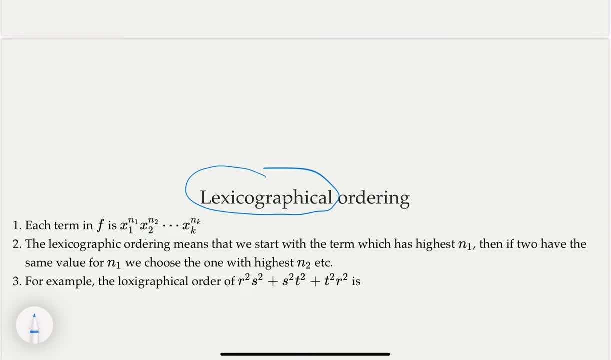 So we need what is called the next-come graphical ordering of the terms. So each term generically is like that, With a portion- you call it Some coefficients see here. But we say that it is in the next-come graphical order if we always start with the highest term, n1, right? 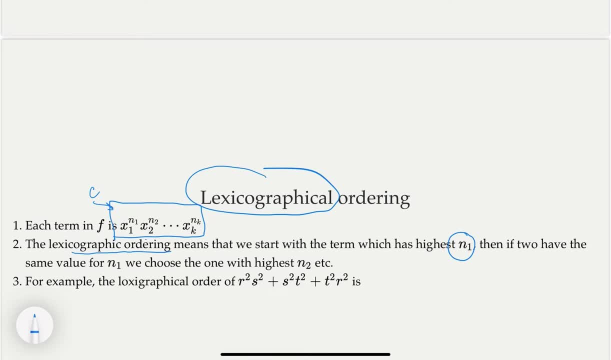 And then if n1 happens to be the same, you know with two terms, and then we're going to choose the highest n2 terms, and so on and so forth, right? So in this example, right, we're going to express it in lexicon: graphical order, right? 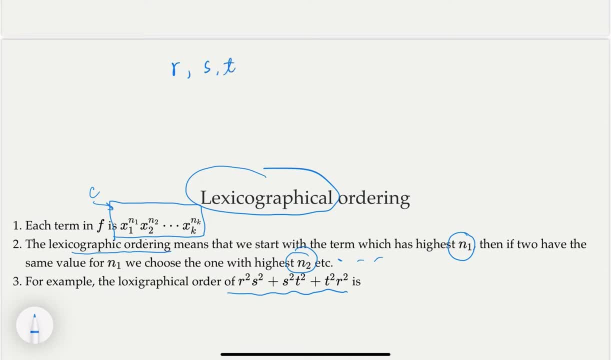 Because, in terms of r, s, t, we're going to use the highest power of r. first. Highest part of r is here and here, right, So we need to write it, And then these two terms, r, squared right, the same thing, and then we're going to compare what is the s power. 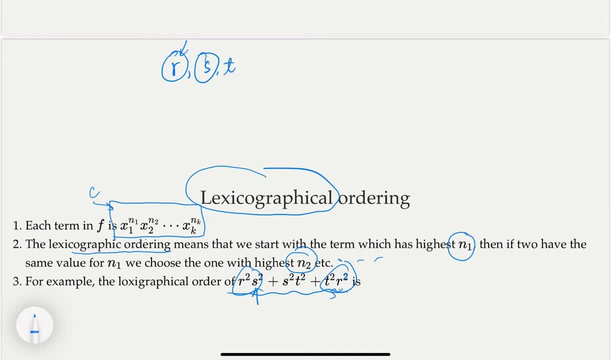 Oh, this one wins because this one is s to the 0th power, this is s to the 2nd power. So the first term would be r squared s squared t to the 0th power. This is the first term here. 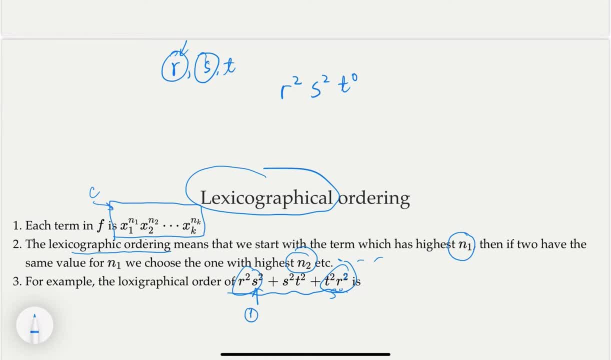 This is the first term, And the remaining one would be this one, because this one has r. This one doesn't have r. So the second term would be r squared right, And s would be 0th power and t to the 2nd power. 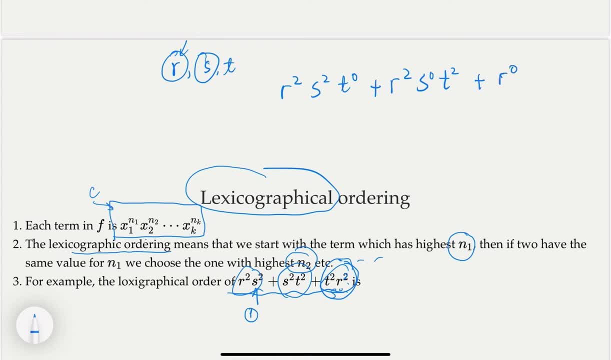 And then, finally, it's going to be r to the 0th power, right, s to the 2nd power, t to the 2nd power. So that is going to be the. Sorry, there's some typo here. 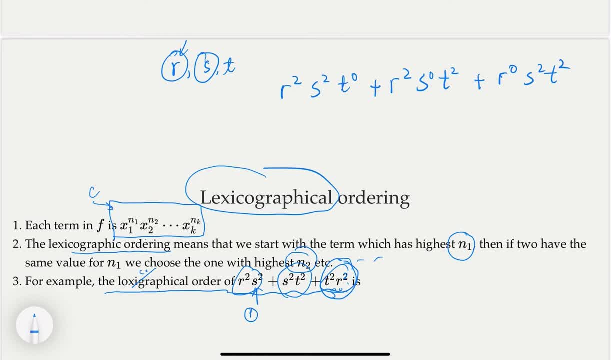 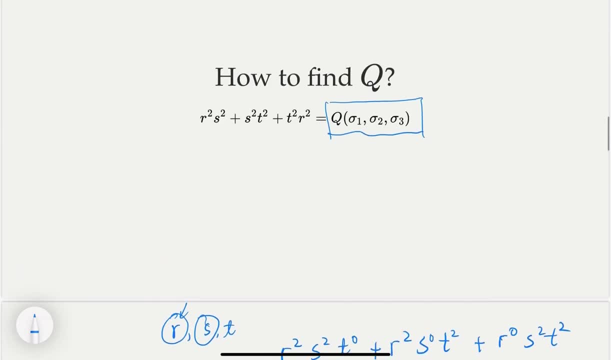 Let's count in a graphical order, all right. So that's, We're going to treat it like that, And then we're going to introduce the algorithm to find this q here, find the polynomial here, right? So how do we do that? 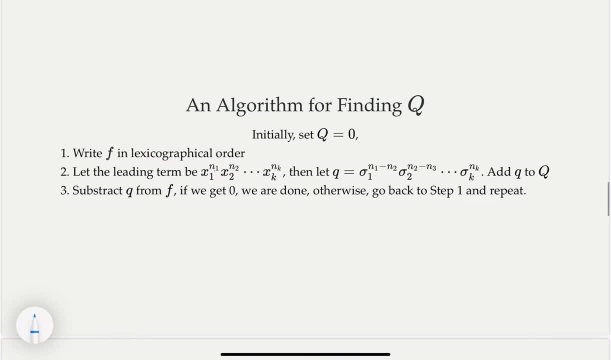 So it turns out that it is an iterative algorithm. So we write f in this order- We already did that earlier- And then assume the leading term. We can look at the leading term right. The leading term earlier would be. in our case would be: 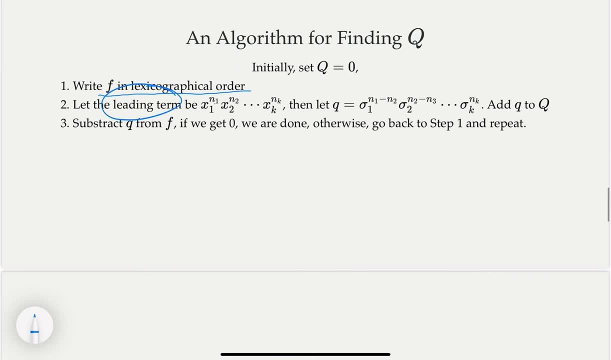 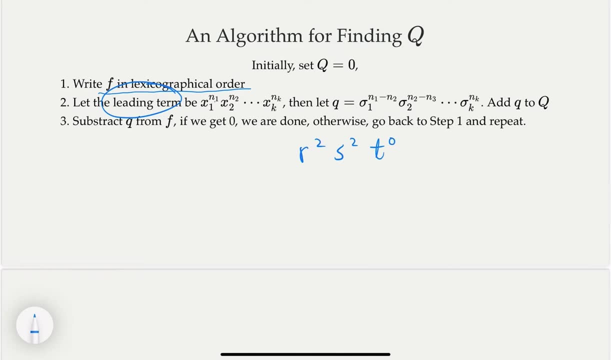 Would be this one. This would be the leading term, right. So it would be r squared s squared t to the 0th power. So in this case, what's n1, n2, nk, right? So n1 would equal 2, n2 equal 2, n3 equal 0, right. 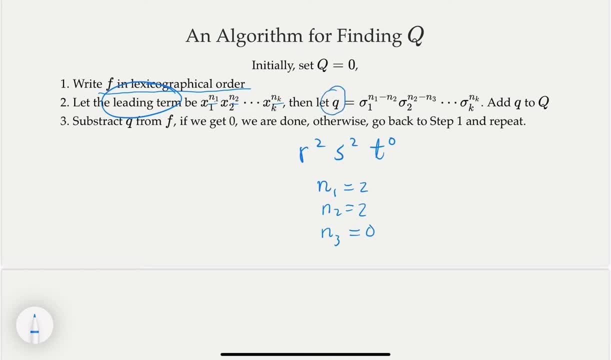 And we're going to define a polynomial in terms of elementary, you know, polynomial here, sigma 1, sigma 2.. In our case, it would be sigma 3, right? So, however, the power would be the difference of the terms. okay. 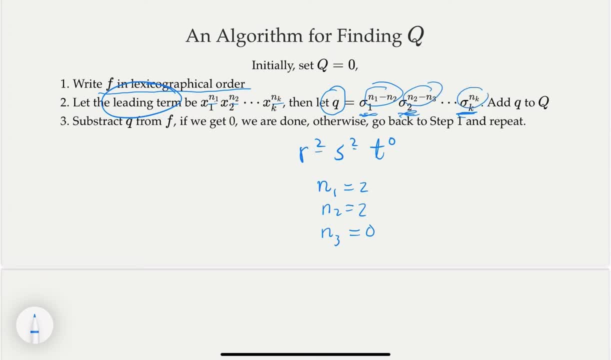 So the difference of the 2 and 2 would be 0.. So the first one would be sigma 1 to the 0th power right, And then sigma 2 would be the 2 minus 0, right n2 minus n3.. 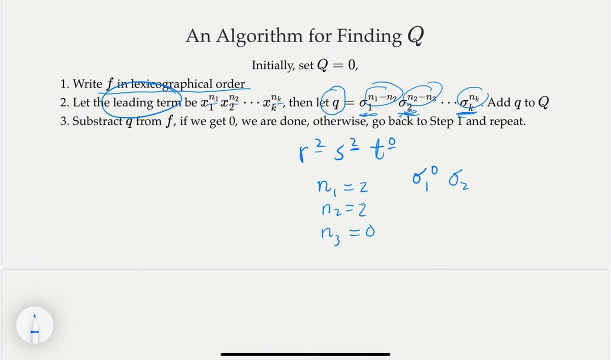 So sigma 2, n2 minus n3, which is 2.. And then sigma 5,. the last term is going to be maintaining the the power. So sigma 3 would be to the 0th power. Now, of course, anything to the 0th power would be equal to 1.. 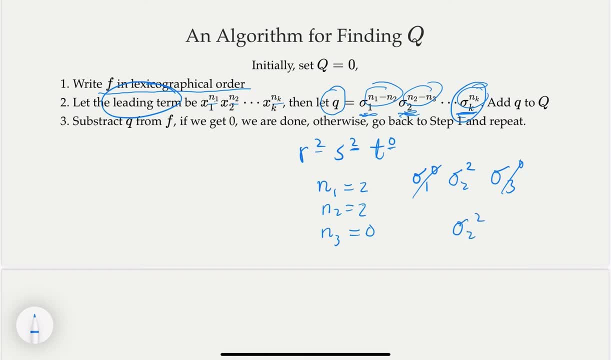 So what we get is sigma 2 squared right. So that's going to be our q right. And then he said: then you subtract q from the original polynomial. If you get a 0, we're done. If not, you're going to go back to step number 1, iterative steps. all right, 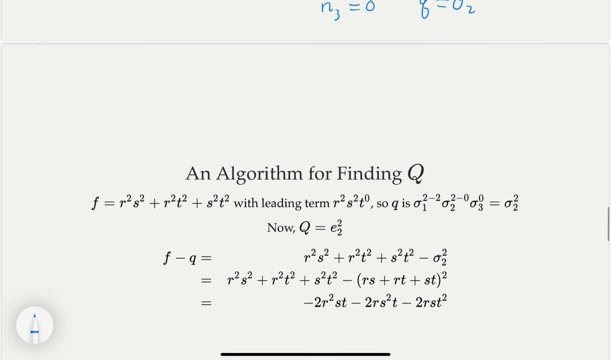 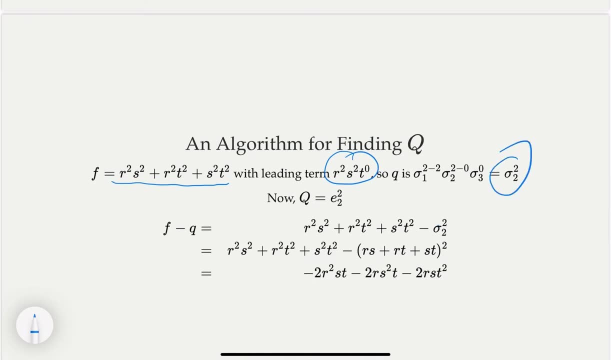 So let's do that. So Our original f is this right. The leading term is, you know, as we look at it earlier. And then we figured out, you know the. you know the term q would be sigma 2, squared right. 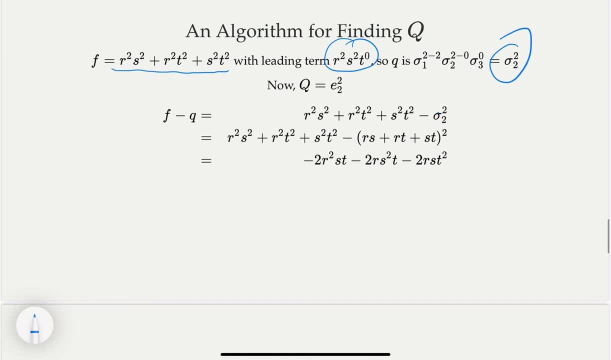 As we did earlier. right, This is the q. So f minus q, you're going to subtract it. This is the original f, right, This is the q. So with subtraction. but what is sigma 2? You know, recall that for a cubic equation, sigma 1 is just r plus f. 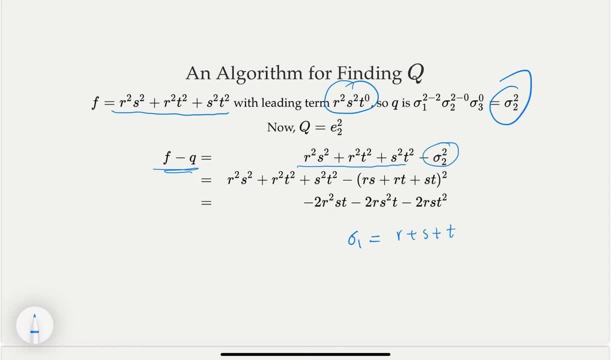 Right, It's just r plus s plus t, And sigma 2 is going to be pairwise sum right: rt plus st And sigma 3 is just rst, right. So just plug in here: right, This is sigma 2.. 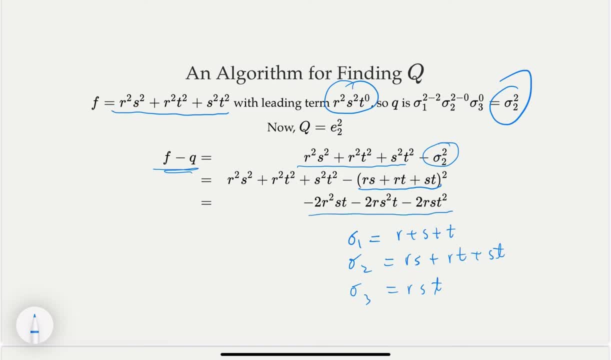 And then if you cancel the term, you get this one right. Okay, So of course, if you spot this, you can notice that there's a common factor. So you can just factor it out And this is going to be rst, right. 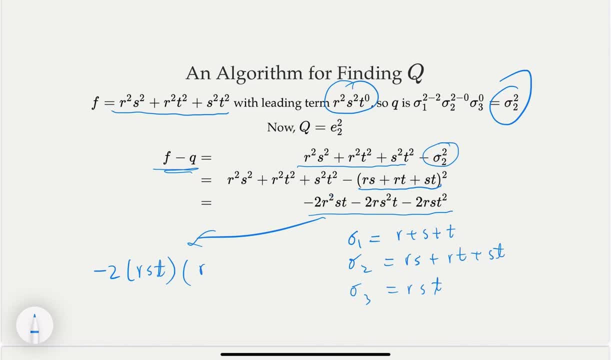 And then the remaining one would be r plus s plus t, And that happens to be sigma 3.. This happens to be the sigma 1, right? So the whole term is like that. Of course, our algorithm does not say that, right. 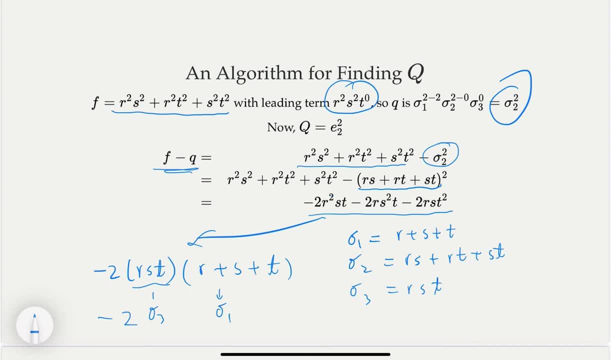 Even though, you know, in our case, we can stop and say: oh, we found the expression in terms of sigma 1 and sigma 3.. But let's follow the algorithm. The algorithm says: look at the remaining. We're going to go back to step number 1, because this is not 0, right? 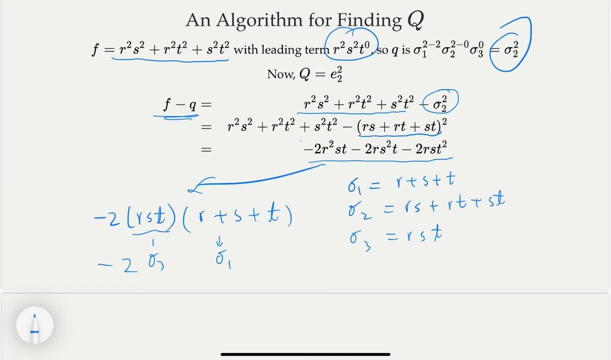 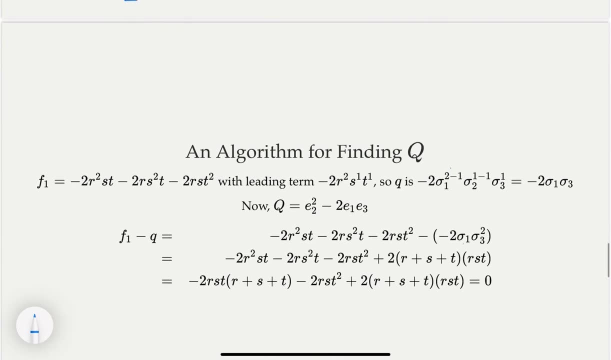 So we're going to go back to the original f And the leading term in this case would be r square st, right Negative 2. r square s is the leading term. So we're going to repeat: Here is the leading term right. 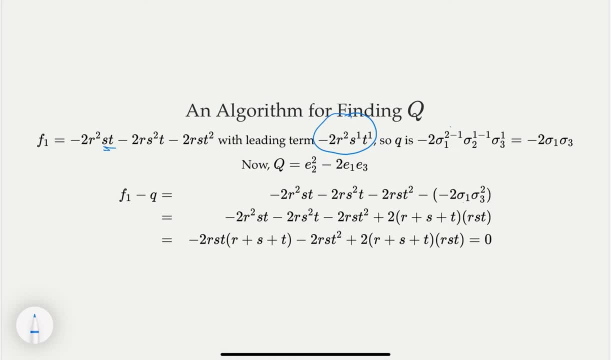 You know rst. here s to the 1th power. So n would be what You know, n1 would be 2.. n2 would be 1.. n3 would be 1.. So the cross-dominant term is co-efficient negative 2.. 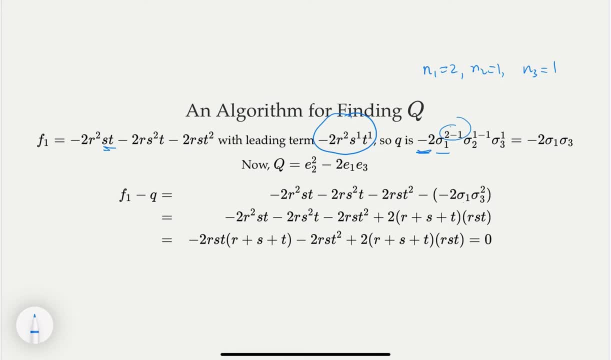 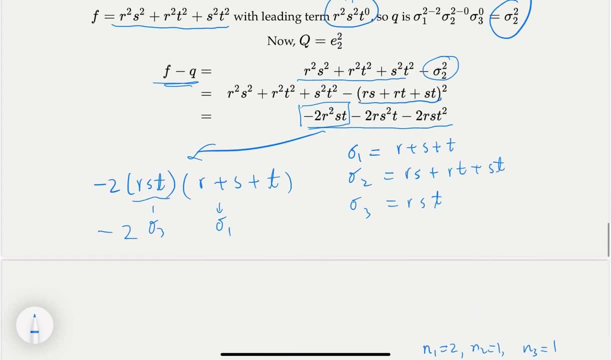 Sigma 1, n1 minus n2 is going to be 1. And this would be 0. This would be 1.. So it turns out to be this one, right, Which is the same as when we looked at it earlier, right. 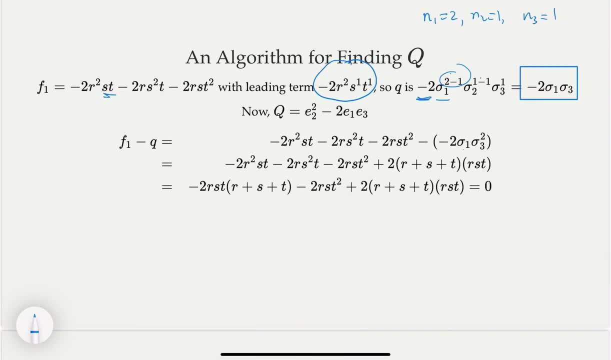 Which is the same thing, right. However, let's follow the algorithm. The algorithm says that you add this to the q. Original q. is this? You're going to add this: negative 2, e1, e3, right? Sorry, this will be sigma. 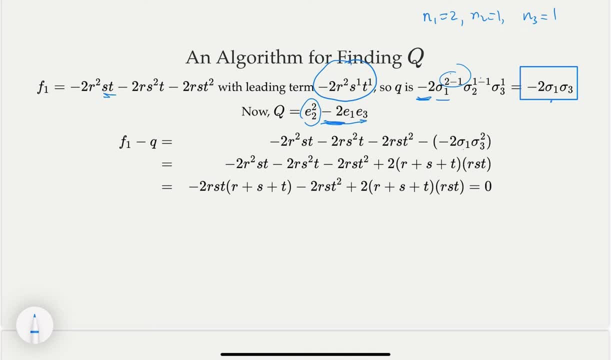 There's a timeout here, Because sometimes people use e to represent the elementary right. In our notation, this would be sigma 2, squared minus 2, sigma 1, sigma 3, right. So let's follow the algorithm. The algorithm says you're going to subtract the q right. 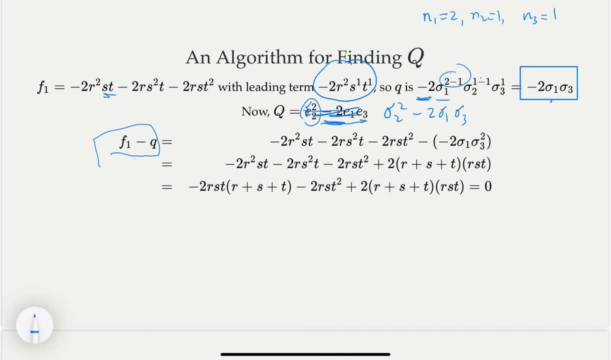 This is our q: You're going to subtract that, right, You're going to subtract that, And then this negative becomes positive, And then this happens to cancel everything: Everything will be 0.. So now you can stop right. So you find the q, which is this one: 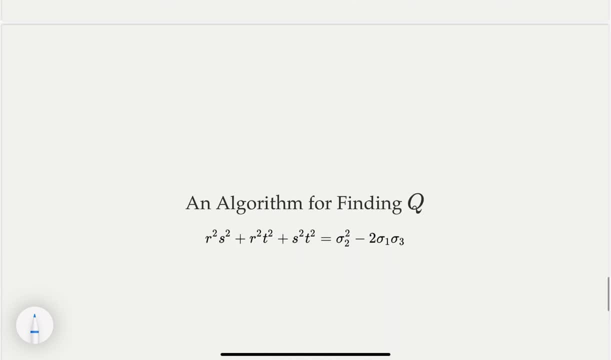 And so, in other words, the conclusion is that this polynomial p or f can be expressed in terms of q, sigma 1, sigma 2, sigma 3.. That is sigma 2 squared minus 2 sigma 1.. sigma 3, right. 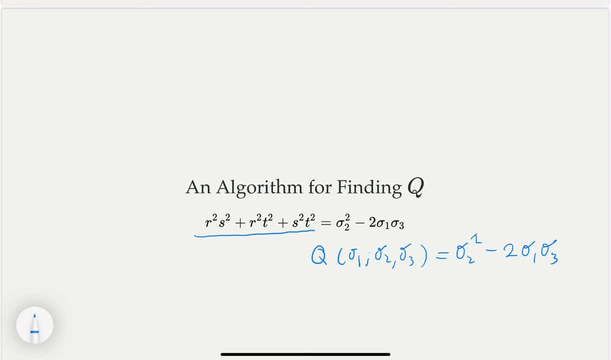 So you can try some other symmetric polynomial using this algorithm. For example, earlier we do the power sum right, Like s3 equal r to the third power plus s to the third power plus t to the third power right, Or s2 equal r squared plus s squared plus t squared right. 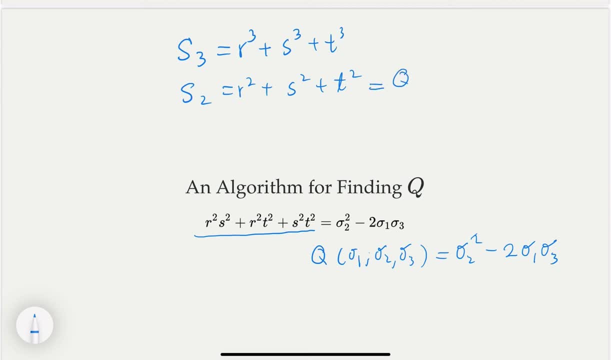 You can find what is corresponding q, right? What is the q here, right? In this case it may be easy because it is actually sigma 1, squared minus 2, sigma 2, right, But you can follow the algorithm and derive the same answer here, right? 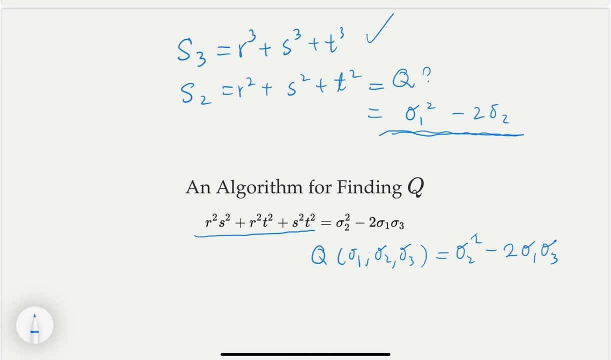 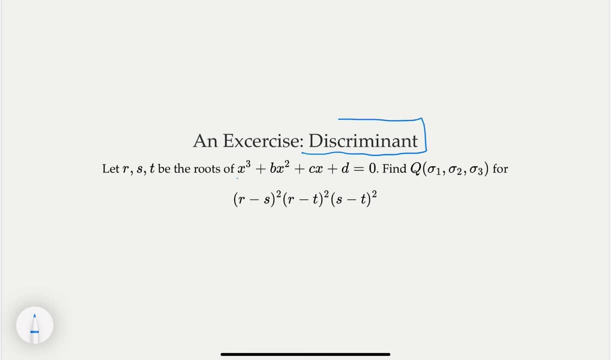 For this one. you can use this as an exercise to figure it out right. As a matter of fact, there's another exercise, which is what is called the discriminant. It's a polynomial right. So for a cubic equation generally, we have b, c, d coefficient, r, c, b, the rules. 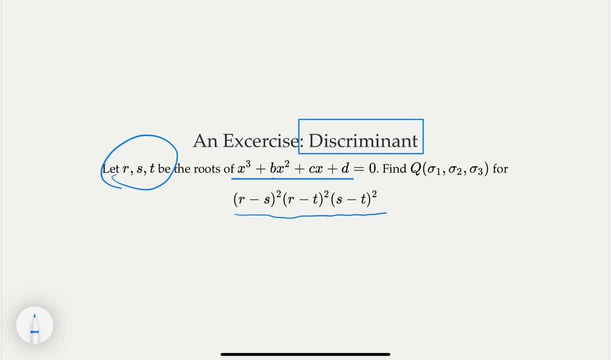 So this is symmetrical right. Let's call this discriminant right. This is delta. It's symmetrical right. And then there must be a q right. You can follow the algorithm to find the q. Notice that when this term equals 0,. 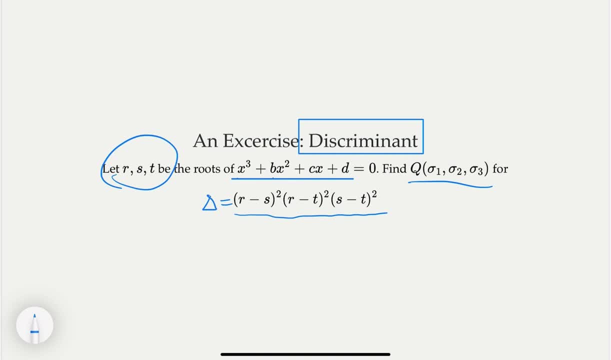 it means what? It means: r minus s or r minus t or s minus t. one of them must be 0, right, At least one of them must be 0. In other words, some rules are identical, So in this case, you may have two identical rules. 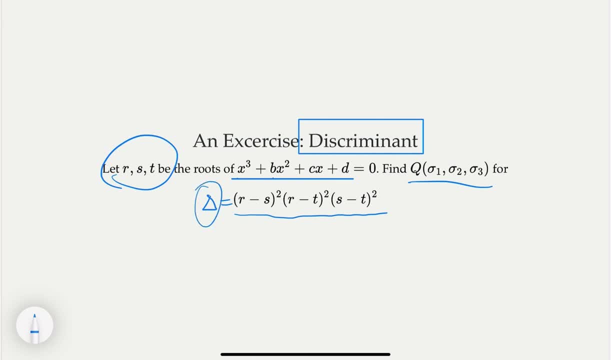 if, and only if, delta discriminant is 0.. Now we leave this as an exercise to find out what is polynomial in terms of sigma 1, sigma 2, sigma 3.. Of course, one thing: you notice that in this case, 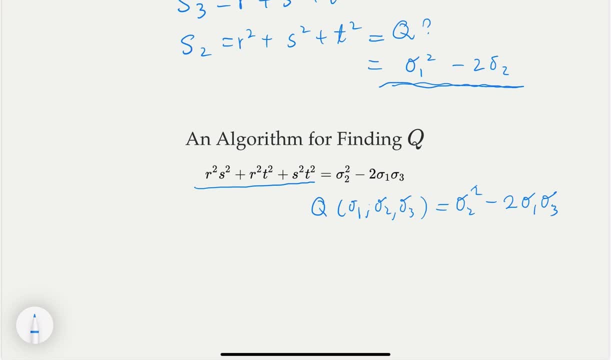 if the equation r is t is for the. if this equation is x to the third, power plus bx, squared plus cx plus d equals 0, earlier we know that. what is sigma 1, right, So sigma 1 would be negative b. 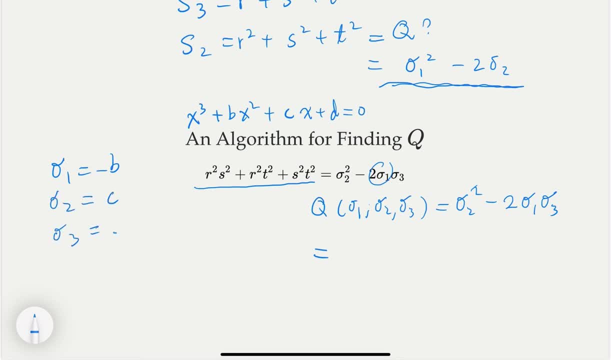 Sigma 2 would equal to c, Sigma 3 would equal negative d right. So in this polynomial you can just plug in and say that this whole thing would equal to sigma 2, which is c squared right, c squared minus 2..